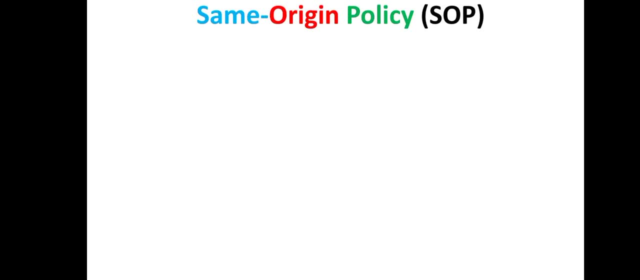 Same origin policy, also abbreviated as SOP, is a security mechanism in web browsers which prevents a malicious website from attacking another unrelated website, So this is an important concept with regards to web application security modeling. Now, this is a web server which is hosting this website. 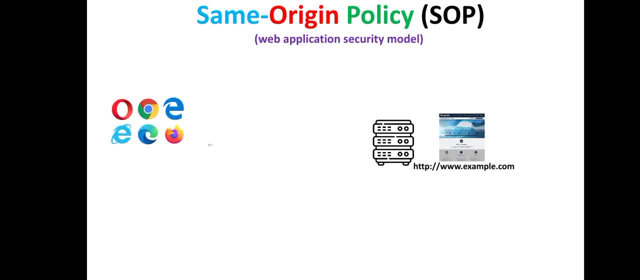 Now a user is using his browser to access this website. Now there is a script which is running on this web page which, upon visit, gets delivered to the web browser of the user, And this script is trying to connect to another web page. Now, if the web browser is compliant with same origin policy, then it will look for the URI, scheme, hostname and port number of second web page. 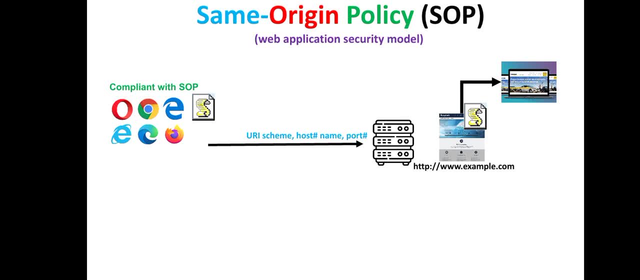 And if it matches with the first And if it matches with the second, Then it will allow access. So in this case, the script is allowed to run on the second web page, since all the parameters are same Now. this same origin policy will provide protections against cross site attacks. 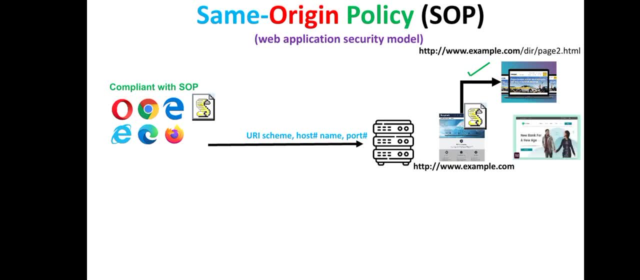 For example, this is a web browser which is running on the second web page. Now, this is a web browser which is running on the second web page. This is a bank website to which a user is already logged in by using his web browser. 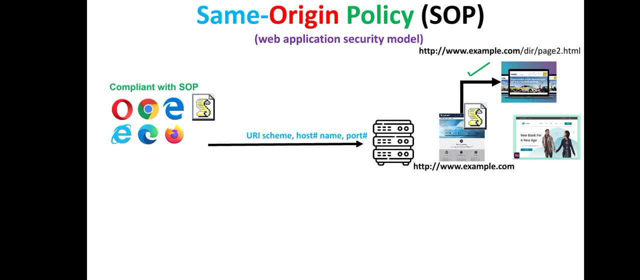 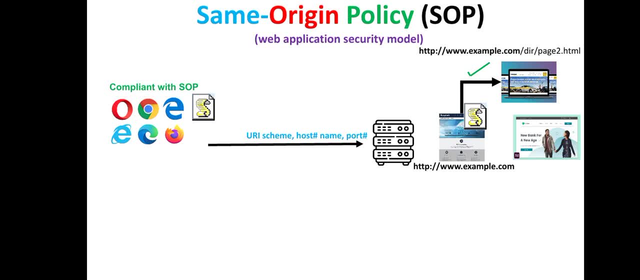 Now this first website is running this malicious script which is trying to perform a cross site request forgery attack by using the credentials of authenticated user. Now, this first website is running this malicious script which is trying to perform a cross site request forgery attack by using the credentials of authenticated user. 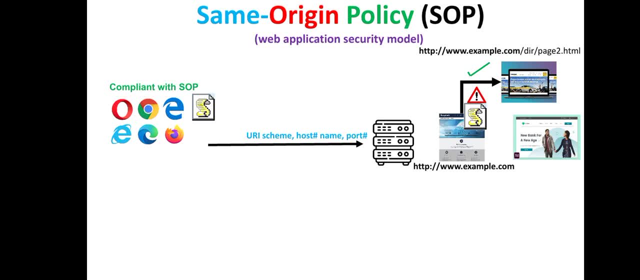 Now this first website is running this malicious script which is trying to perform a cross site request forgery attack by using the credentials of authenticated user. Now, this first website is running this malicious script which is trying to perform a cross site request forgery attack by using the credentials of authenticated user. 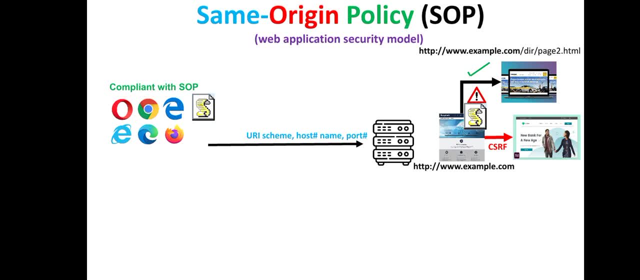 Now this first website is running this malicious script which is trying to perform a cross site request forgery attack by using the credentials of authenticated user. Now, this first website is running this malicious script which is trying to perform a cross site request forgery attack by using the credentials of authenticated user. 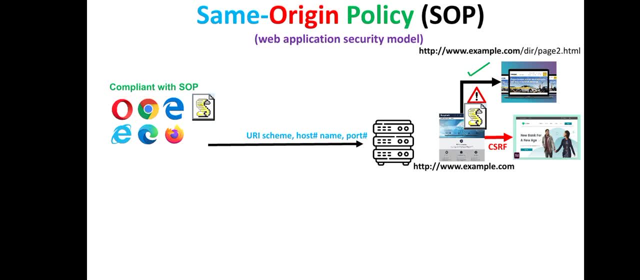 Now this first website is running this malicious script which is trying to perform a cross site request forgery attack by using the credentials of authenticated user. Now, this first website is running this malicious script which is trying to perform a cross site request forgery attack by using the credentials of authenticated user. 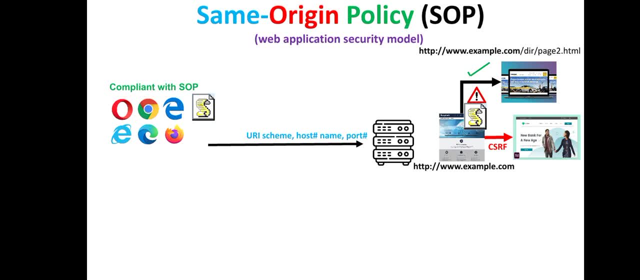 Now this first website is running this malicious script which is trying to perform a cross site request forgery attack by using the credentials of authenticated user. Now, this first website is running this malicious script which is trying to perform a cross site request forgery attack by using the credentials of authenticated user. 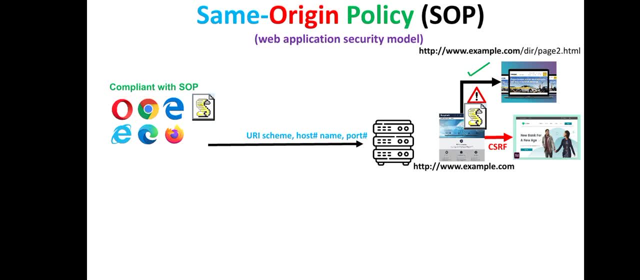 Now this first website is running this malicious script which is trying to perform a cross site request forgery attack by using the credentials of authenticated user. Now, this first website is running this malicious script which is trying to perform a cross site request forgery attack by using the credentials of authenticated user. 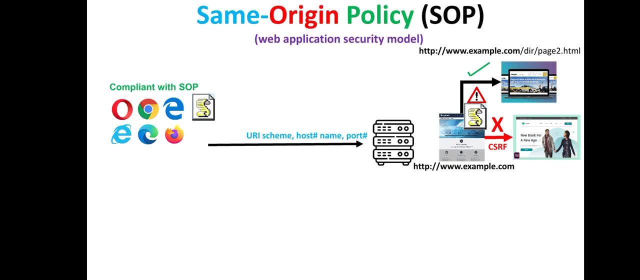 Now this first website is running this malicious script which is trying to perform a cross site request forgery attack by using the credentials of authenticated user. Now, this first website is running this malicious script which is trying to perform a cross site request forgery attack by using the credentials of authenticated user. 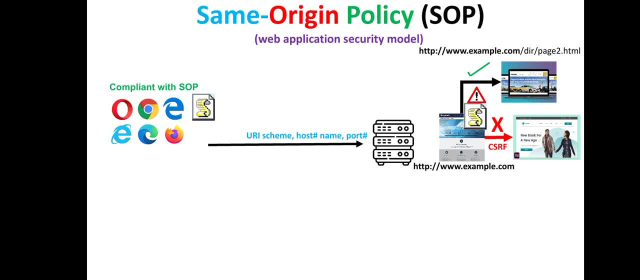 Now this first website is running this malicious script which is trying to perform a cross site request forgery attack by using the credentials of authenticated user. Now, this first website is running this malicious script which is trying to perform a cross site request forgery attack by using the credentials of authenticated user. 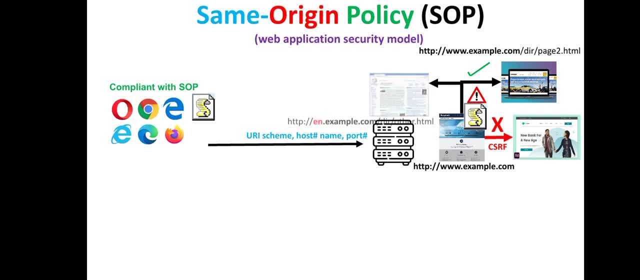 Now this first website is running this malicious script which is trying to perform a cross site request forgery attack by using the credentials of authenticated user. Now, this first website is running this malicious script which is trying to perform a cross site request forgery attack by using the credentials of authenticated user. 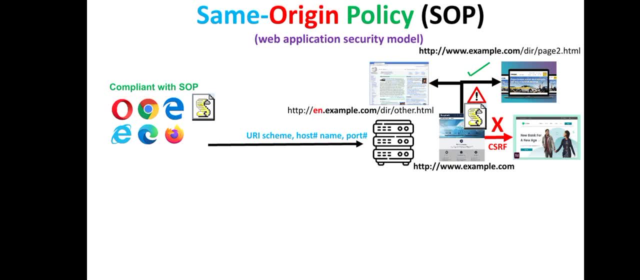 Now this first website is running this malicious script which is trying to perform a cross site request forgery attack by using the credentials of authenticated user. Now, this first website is running this malicious script which is trying to perform a cross site request forgery attack by using the credentials of authenticated user. 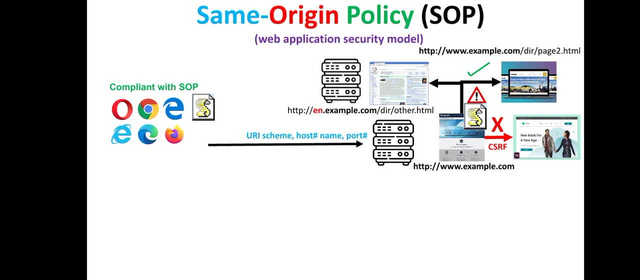 Now this first website is running this malicious script which is trying to perform a cross site request forgery attack by using the credentials of authenticated user. Now, this first website is running this malicious script which is trying to perform a cross site request forgery attack by using the credentials of authenticated user. 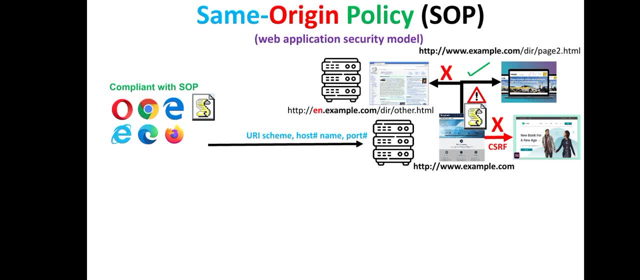 Now this first website is running this malicious script which is trying to perform a cross site request forgery attack by using the credentials of authenticated user. Now, this first website is running this malicious script which is trying to perform a cross site request forgery attack by using the credentials of authenticated user. 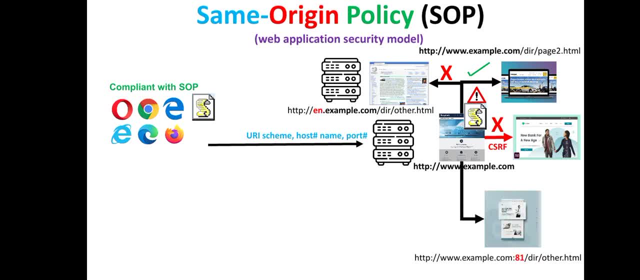 Now this first website is running this malicious script which is trying to perform a cross site request forgery attack by using the credentials of authenticated user. Now, this first website is running this malicious script which is trying to perform a cross site request forgery attack by using the credentials of authenticated user. 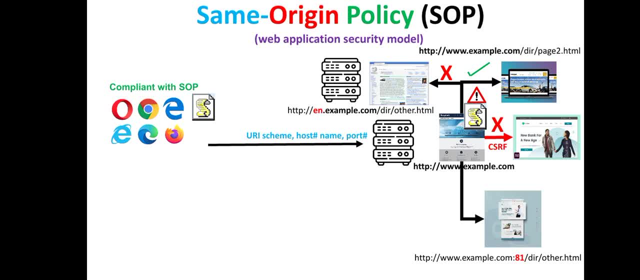 Now this first website is running this malicious script which is trying to perform a cross site request forgery attack by using the credentials of authenticated user. Now, this first website is running this malicious script which is trying to perform a cross site request forgery attack by using the credentials of authenticated user. 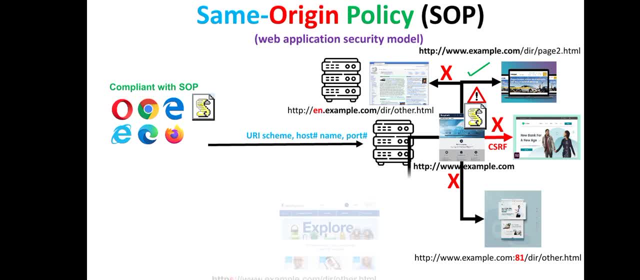 Now this first website is running this malicious script which is trying to perform a cross site request forgery attack by using the credentials of authenticated user. Now, this first website is running this malicious script which is trying to perform a cross site request forgery attack by using the credentials of authenticated user. 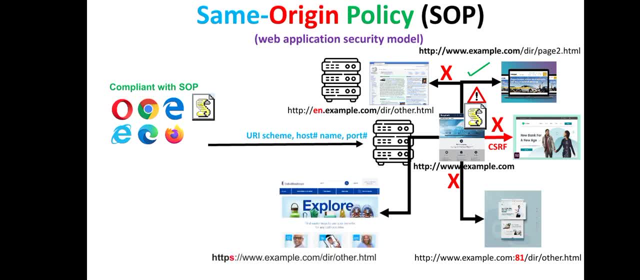 Now this first website is running this malicious script which is trying to perform a cross site request forgery attack by using the credentials of authenticated user. Now, this first website is running this malicious script which is trying to perform a cross site request forgery attack by using the credentials of authenticated user. 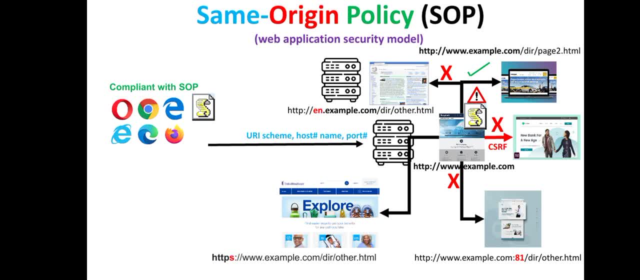 Now this first website is running this malicious script which is trying to perform a cross site request forgery attack by using the credentials of authenticated user. Now, this first website is running this malicious script which is trying to perform a cross site request forgery attack by using the credentials of authenticated user. 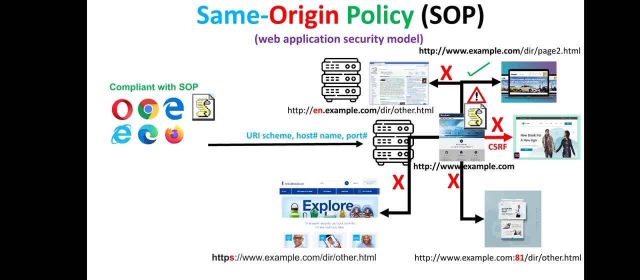 Now this first website is running this malicious script which is trying to perform a cross site request forgery attack by using the credentials of authenticated user. Now, this first website is running this malicious script which is trying to perform a cross site request forgery attack by using the credentials of authenticated user. 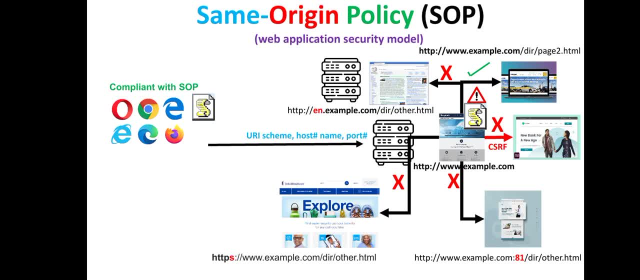 Now this first website is running this malicious script which is trying to perform a cross site request forgery attack by using the credentials of authenticated user. Now, this first website is running this malicious script which is trying to perform a cross site request forgery attack by using the credentials of authenticated user.